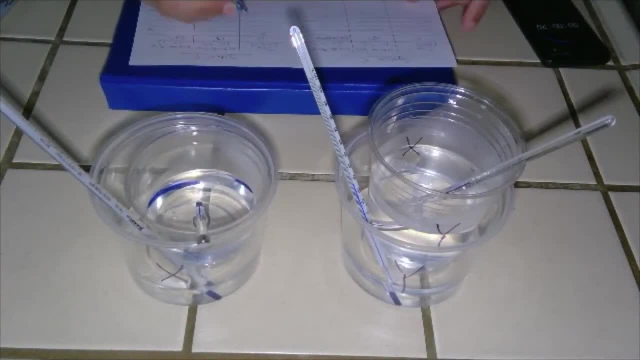 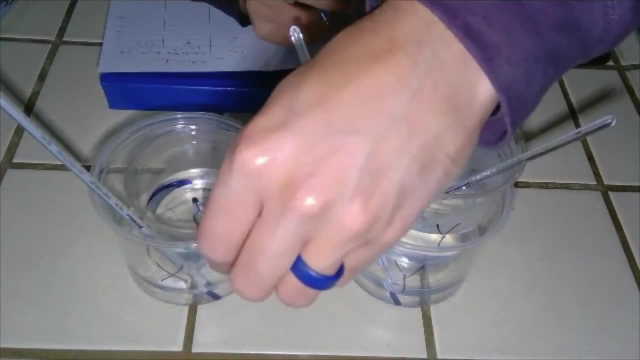 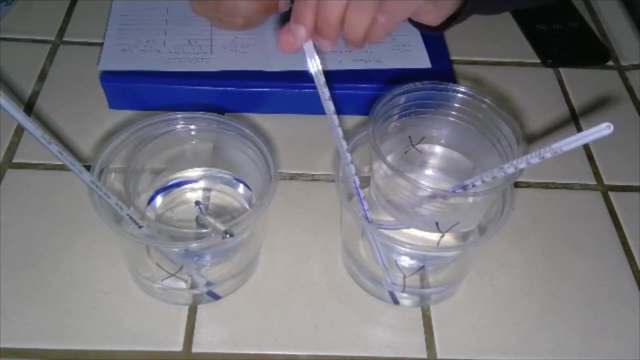 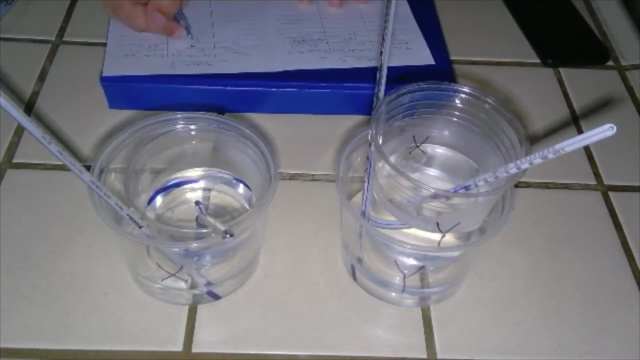 Okay, So at five minutes it's about 23 degrees Celsius And the inside of the cup is at 30 degrees Celsius And the outside of the cup for Y is at 28 degrees Celsius, But the inside of the cup is at 30 degrees Celsius. 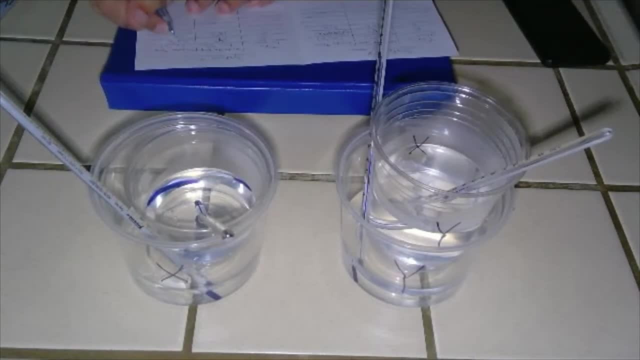 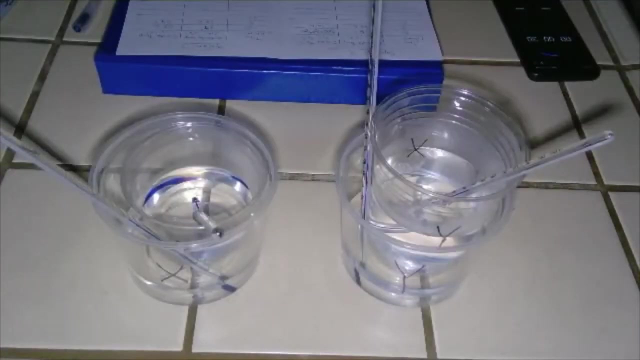 And the inside of the cup for Y is at 24 degrees Celsius, And then we're going to go ahead and set the timer for another five minutes and we'll see what happens A few minutes later. All right, So that's been about five minutes. I'm going to take another measurement of the 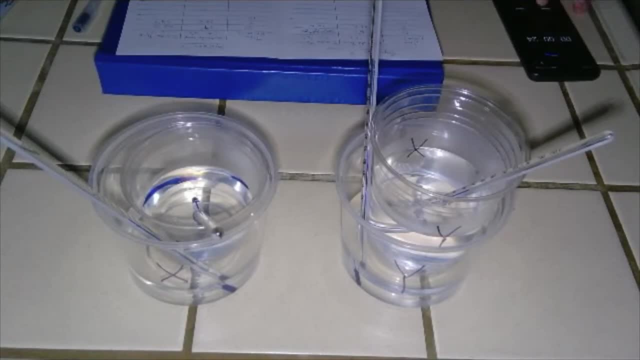 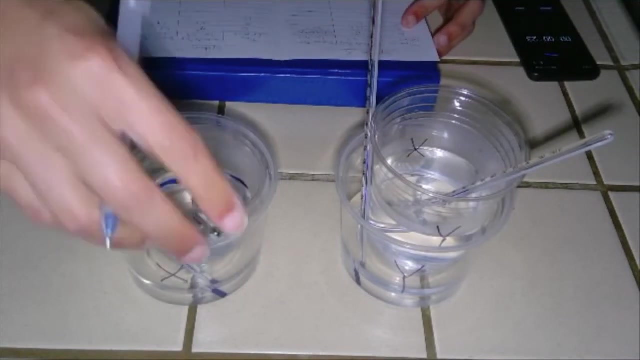 temperature. Okay, So now we're going to take another measurement of the temperature. The outside temperature of the cold water of X is at around 26 degrees Celsius, And the inside temperature is at 29 degrees Celsius. All right, I'm going to go back to record. 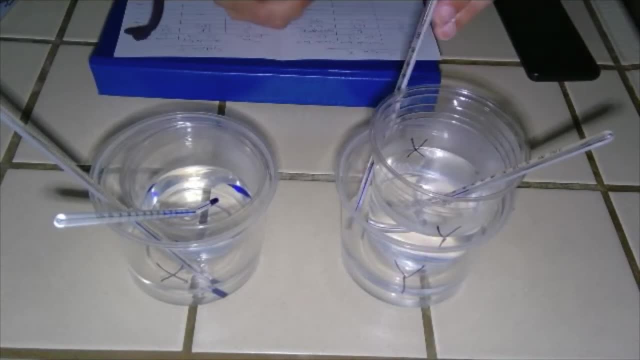 Okay, And the outside X is at 30 degrees Celsius and the inside temperature is at 33, 33 degrees Celsius. So we're going to check at another 5 minute interval and what you should see is that the water samples inside and outside the cup are going to be reaching equilibrium. so where? 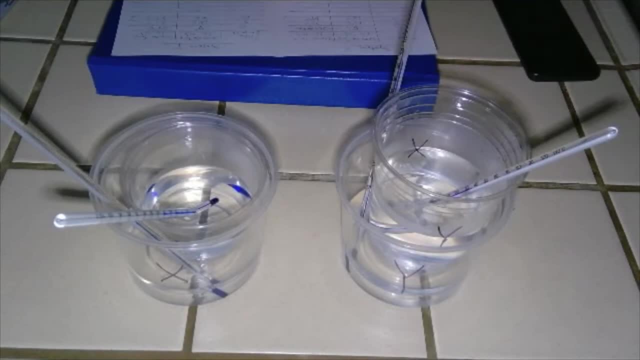 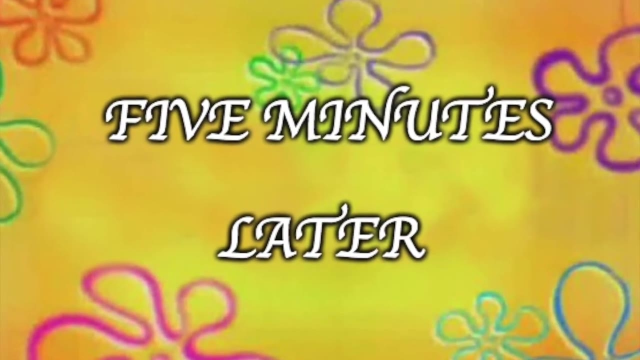 the temperatures are the same, The average kinetic energy inside and outside is the same, So we'll revisit our data in just a few, A few minutes later. Okay, we're going to go ahead and take one more measurement of our temperatures in our 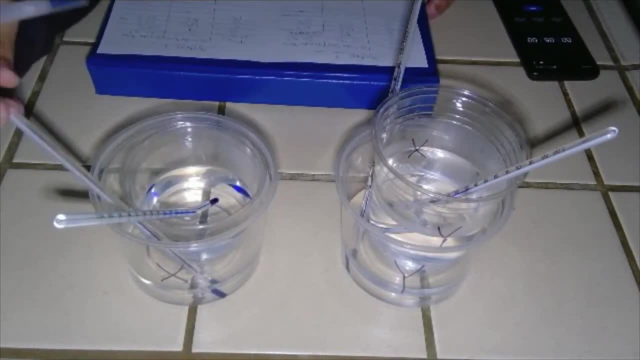 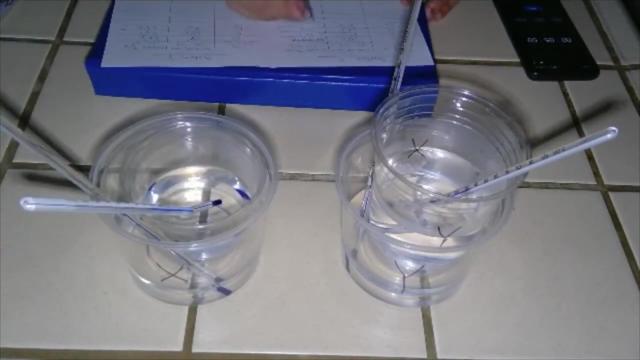 systems. Let's take a look at system X. The outside temperature is 20 degrees Celsius, 27 degrees after 15 minutes, 27 degrees, And the inside temperature is at 29 degrees 29 degrees Celsius And if we take a look at the outside temperature here, it's 30, 31 degrees Celsius. 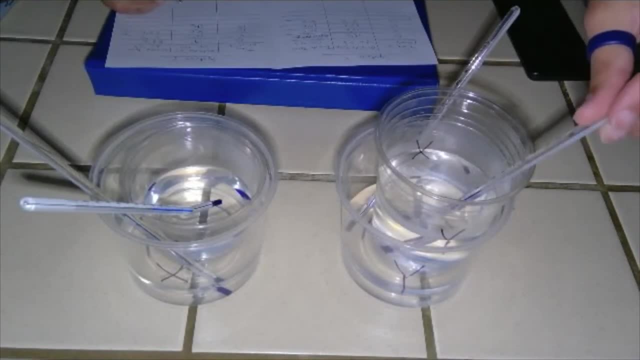 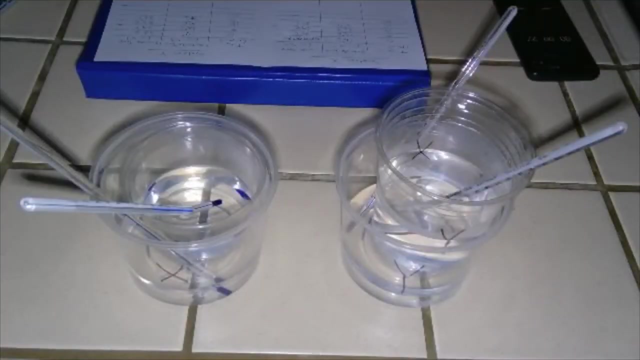 And our inside temperature. Inside temperature for Y is 33.. And we'll take one more look at our temperature in 5 minutes to see if it has reached. if either system has reached equilibrium A few minutes later. All right, so we're going to take our final measurement of temperature. 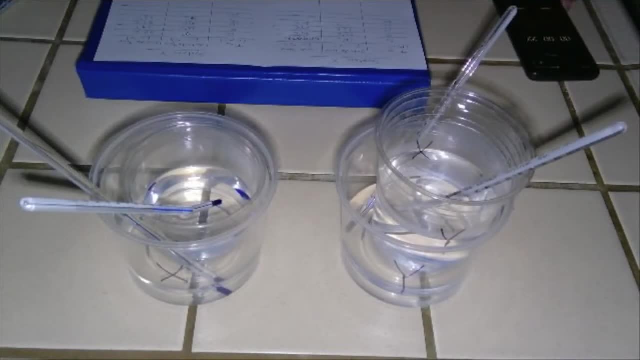 For our equilibrium test. So let's take a look at system X Now. system X is at 27 degrees Celsius, outside the cup, 27 degrees Celsius, And the inside of the cup is also at 27 degrees Celsius. Okay, And we'll take a look at the outside. 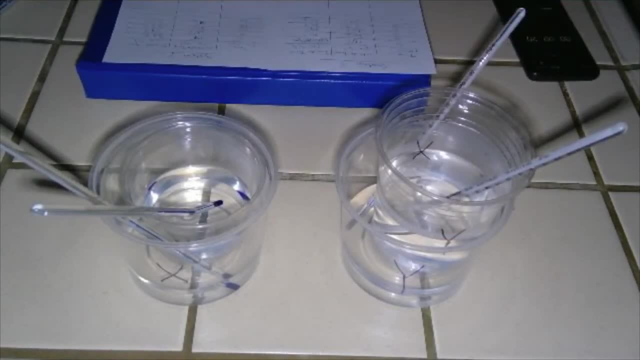 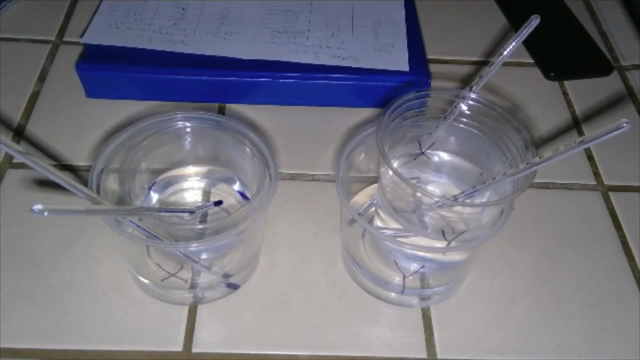 The outside cup here is at 30 degrees Celsius- say, 30.5 degrees Celsius- and the inside temperature is equal to 32 degrees Celsius. So let's take a look at this data. Okay, So this data tells us some important things. 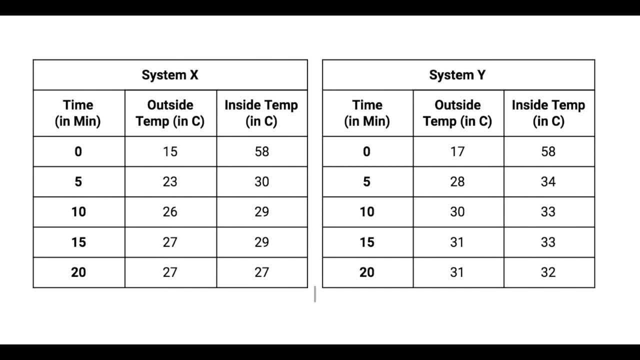 Both systems were able to reach equilibrium, but system X reached equilibrium at 27 degrees Celsius and system Y reached equilibrium at around 31, 32 degrees Celsius. Why did cup Y and container Y end with a higher equilibrium temperature than cup X and container? X.